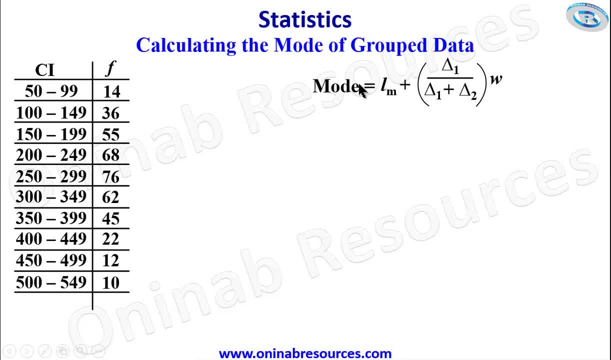 grouped data. So we have our formula here. Lm is the lower class boundary of the modal class and the delta one is the positive difference between the frequency of the modal class and the frequency of the class before it, While delta two is the positive difference between the frequency of the modal class and the frequency of the class after. 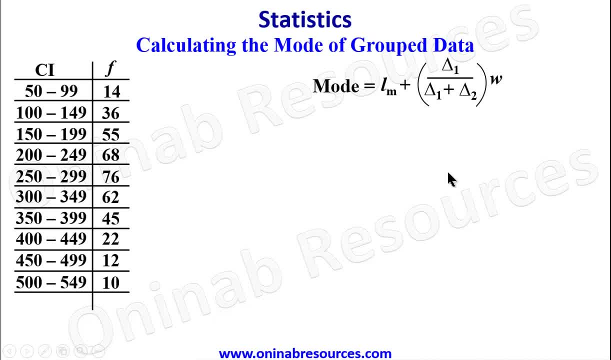 it. We still have our w as the class width or class size of the modal class. So we are going to create additional column to the table to accommodate the lower class. So we have our boundary, So we have additional column as lower class boundary And again we are going to make 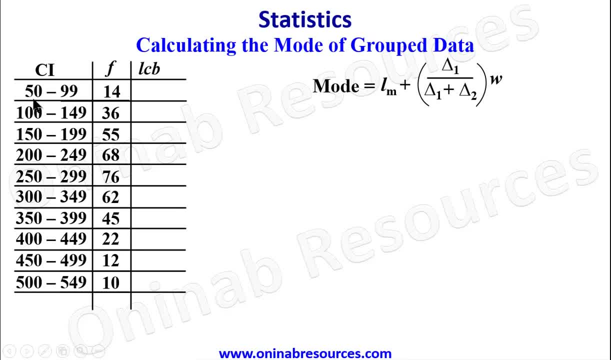 use of only the lower limits of the respective class intervals. So we make use of this lower limit. This is the upper limit. For your information, if there is a class interval before the first class interval, the upper class interval will be 49.. So we are going to. 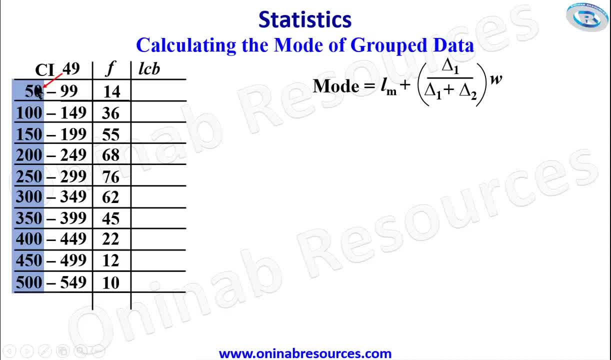 make use of this 49 and 50 to get the lower class boundary of the first class interval. So we say 49 plus 50 divided by 2, which gives 49.5.. Then again we go with 99 and 100.. 99 plus 100 divided by 2. 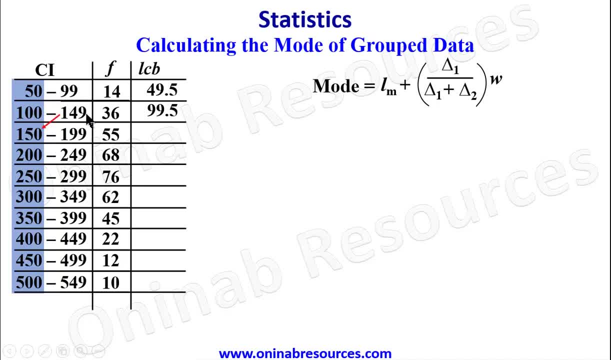 gives 99.5.. Then 149 and 150.. Adding them and divide by 2, we have 149.5.. 199 and 200.. Adding and dividing by 2, we have 199.5.. Then also 249 and 250.. 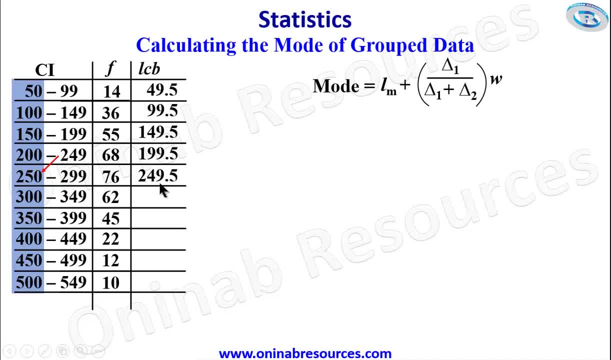 Adding them and dividing by 2, we have 249.5.. 299 and 300.. Adding them and divide by 2 gives 299.5.. 349 and 350.. The sum divided by 2 gives 349.5.. 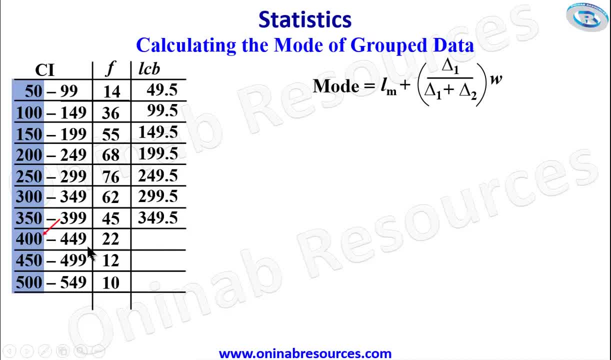 399 plus 400 divided by 2 gives 399.5.. 449 plus 450 divided by 2 gives 449.5.. Then 499 plus 500 divided by 2 gives 499.5.. So, having gotten this, we then go ahead. 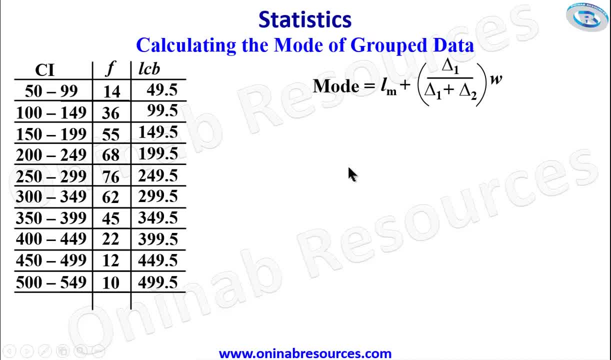 to identify the modal class. The modal class will be obtained via the frequency column, by identifying the highest frequency, and the highest frequency here is 76. So the class interval to it will give us the modal class interval. So this is the modal class interval. So it is very obvious now that our lm is. 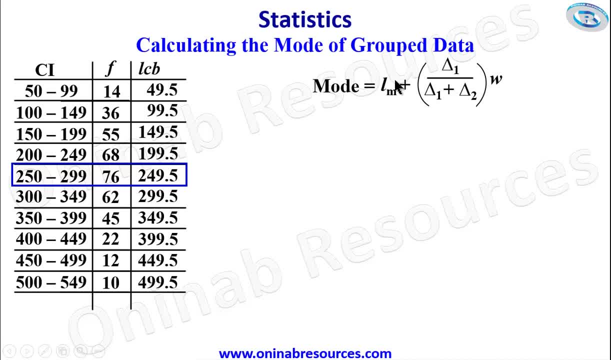 249.5.. We can then go ahead to calculate delta 1, delta 2 and w. Our delta 1 is the positive difference between the frequency of the modal class and the frequency of the class before it, which is 76 and 68. So we have to find the. we then find the positive difference, which is 76 minus 61.. 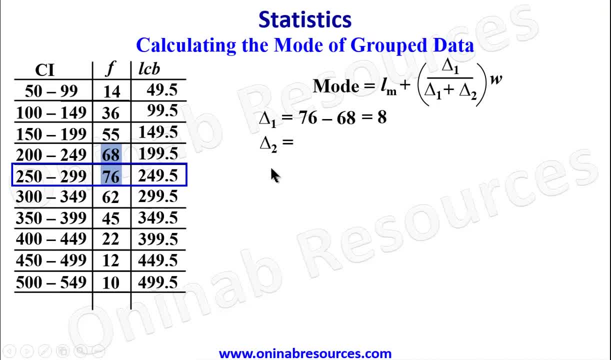 which gives 8. then for Delta 2, it is going to be the frequency of the moda class and the class after each. so we find the difference between the two frequencies. that's going to give us 76 minus 62 and that gives 14 and our class. 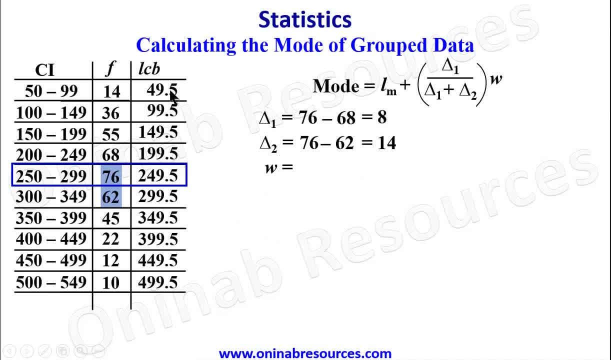 weeks, which is the W. this is equal class interval. we have a quad class interval here, since ninety nine point five minus forty. nine point five gives fifty one. forty nine point five minus tilt. nine point five gives 50 moonlight admin point five minus one. forth nine point five gives fifty. in the same way, 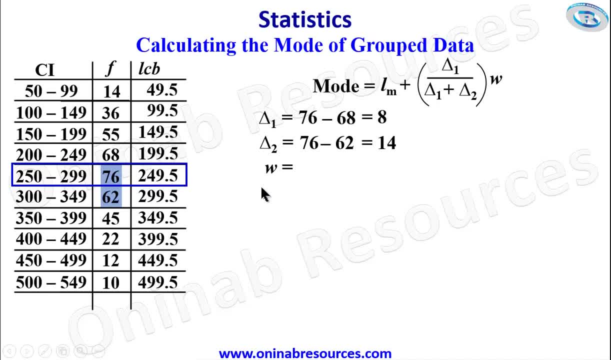 249 point five minus one. ninety nine point five gives fifty. therefore, because of our class interval at X, which gives the CoronaIG temporarily 1 flying, one class size is 50. then we've gotten all the parameters needed to calculate the mode so that our mode now will be equal to our LM. our LM here is the lower class. 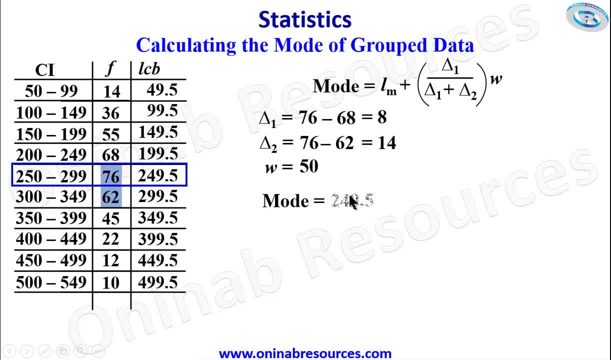 boundary of the model class, that is 249.5 plus Delta 1. Delta 1 is 8, so I have an 8 over 8 plus 14. since Delta 1 is 8, 14 is Delta 2. then multiply by a class. 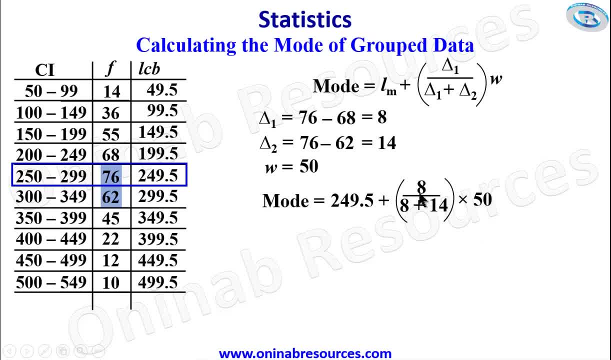 width, which is 50. so again we are going to simplify the brackets. then multiply by 50, so we now have 249 point 5 plus 18 point 1, 8 to 2 decimal places. you now have 8 over 8 plus 14, so we multiply by a class width, which is 50, so we now have 249 point 5 plus 18 point one. 8 to 2 decimal places. 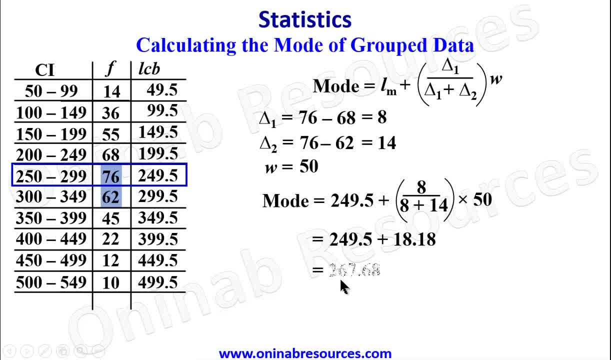 then, summing up this, we have 267.68 as the mood. i hope you love this. you enjoy the class. thank you for watching. please remember to like and share this video. don't forget to subscribe to our youtube channel. also check the description section of this video on our youtube channel. 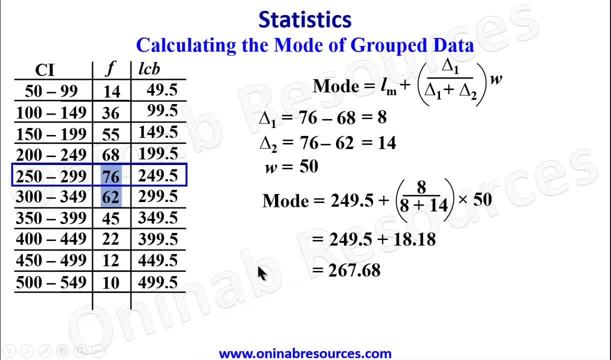 to get the other videos on statistics. until we come your way again, goodbye. 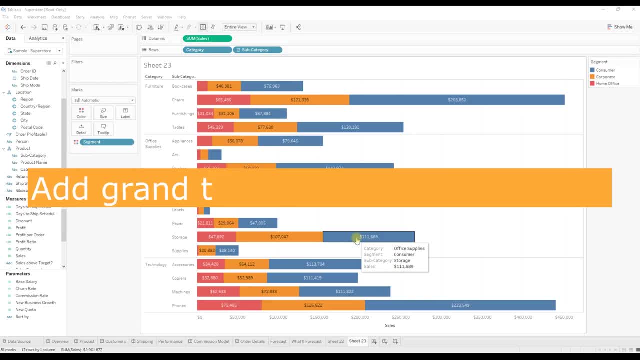 Hi, in this video I will show you how to add grand totals in a slag bar chart. In this view we have sum of sales showing by category and subcategory and each color represents a segment To add a grand total generally we go to analysis and then select total and 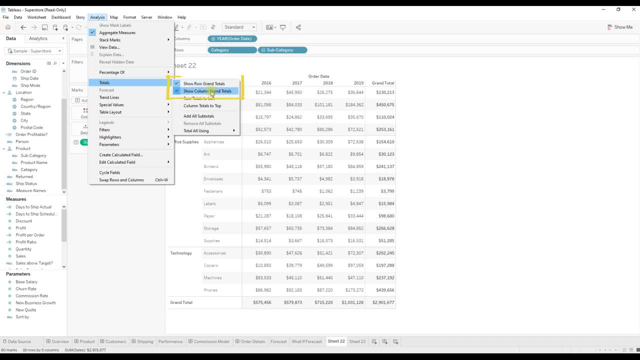 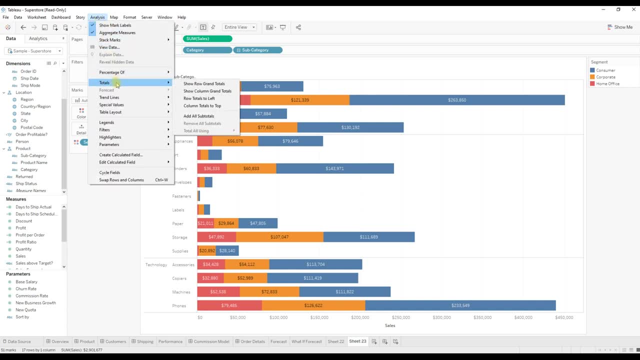 from here, we will add grand totals by row or column. So if you do the same thing in the slag bar chart, you don't see the grand totals applied. See, we don't have grand totals. Okay, so that's why you need to use reference lines. To add a reference line, you need to. 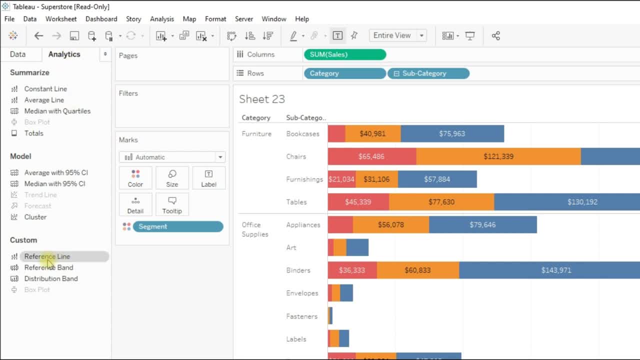 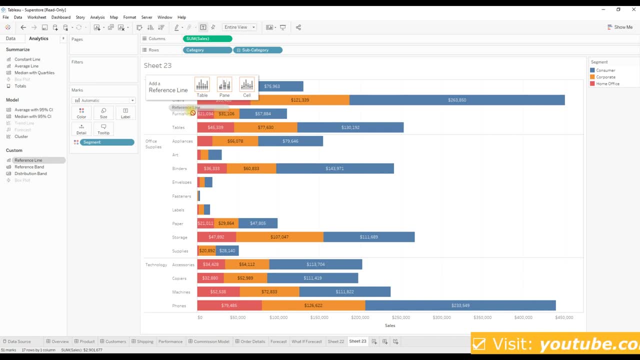 go to analytics tab and then drag reference line to the view. As soon as you drag reference line to the view, you will see a reference line You can drag and drop onto the view. You have three options here. You can drag on the table or